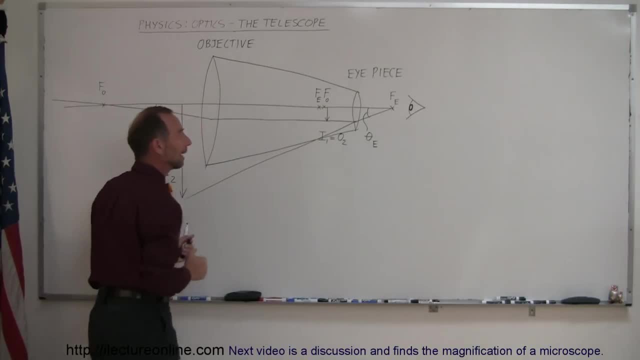 right here, which is a virtual image on the same size as the object, and that then offers the magnification of the telescope. So the magnification of this telescope is simply the ratio of the angle formed by the image of the second lens divided by the angle formed by the 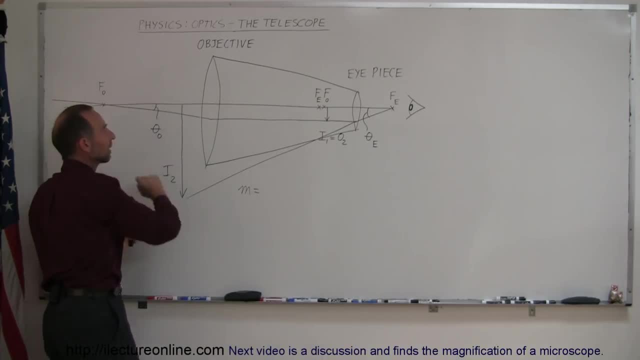 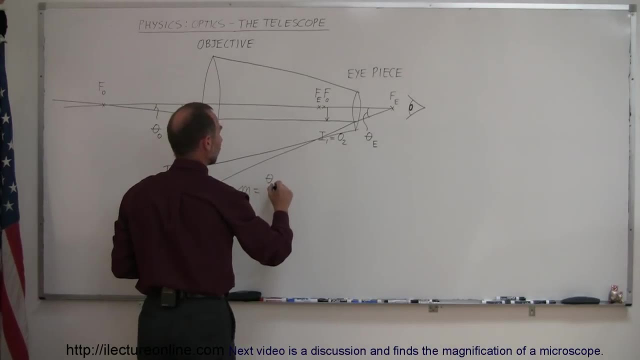 object coming into the first lens. So this would be the angular size of the object, and this would then be the angular size of the second image, which is the image that the observer looks at. So this would be equal to theta sub e divided by theta sub o, the theta caused by the object. 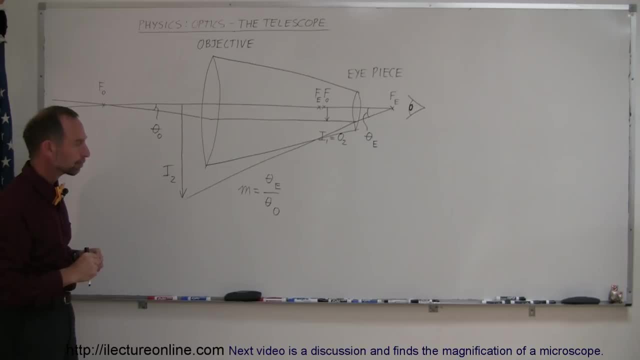 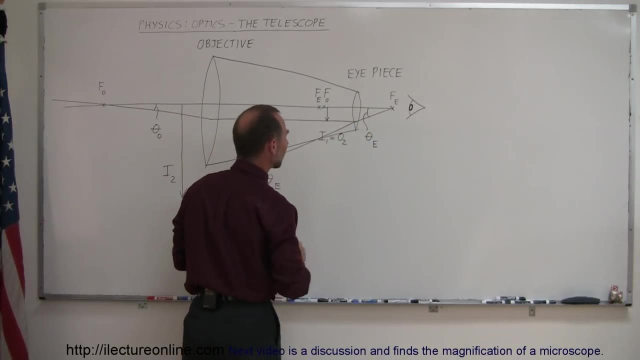 the theta caused by the eyepiece. looking at the final image, Okay, now we can say that for small angles the angle theta is equal to the tangent of that angle theta, and the definition of tangent is opposite side over adjacent. So the angular size of the image formed by the eyepiece can be defined as the height of the image here formed by the first. 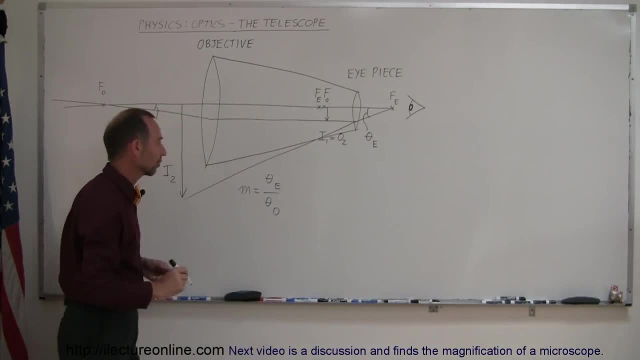 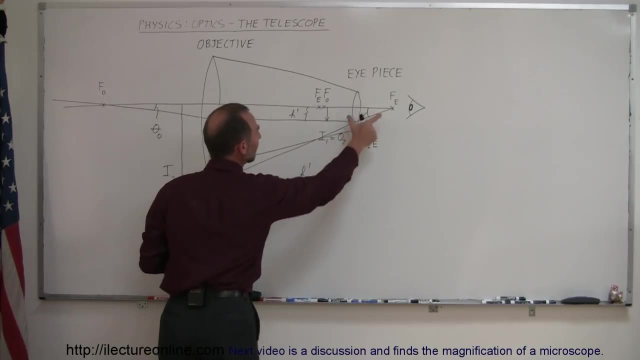 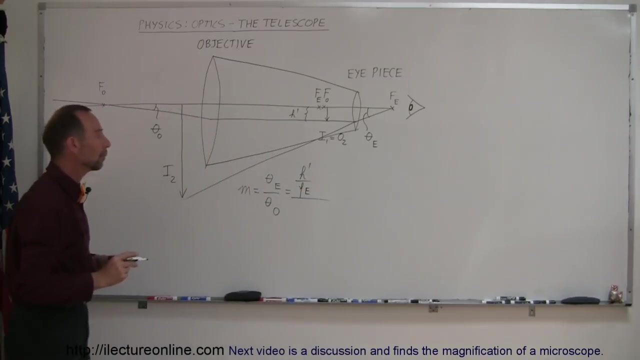 lens divided by the focal distance of the second lens. So this is equal to the height of the image, h, so h prime. let's call this h prime and divide that by the distance to the focal point. that would be f sub e, That would be the focal length right there, and we divide that by the angular size of. 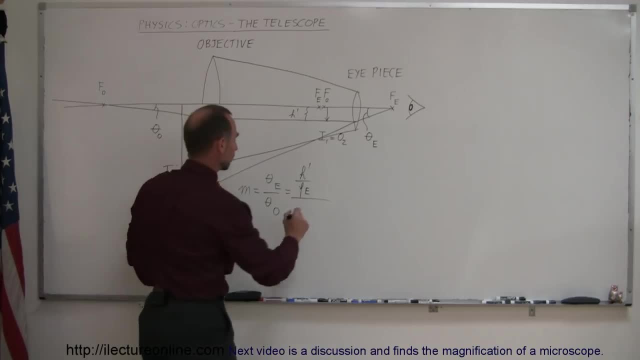 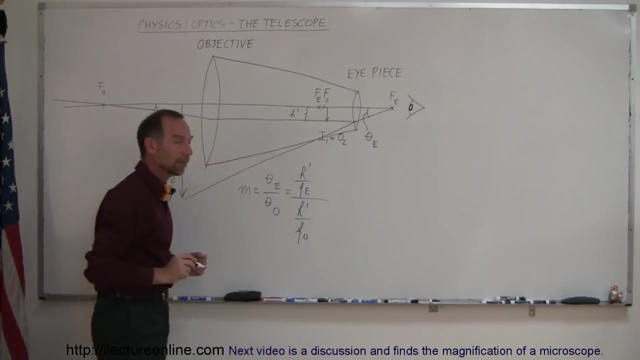 the object, which would be the height of the image right here, which is h prime, divided by the focal length of the objective lens, which is f sub o. All right, now we have two fractions divided by one another, so this can be written as a product of h prime- o. 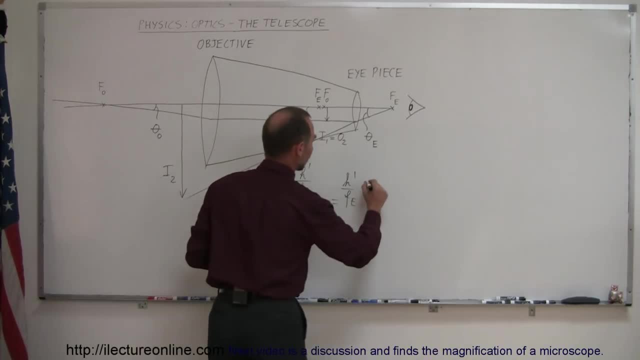 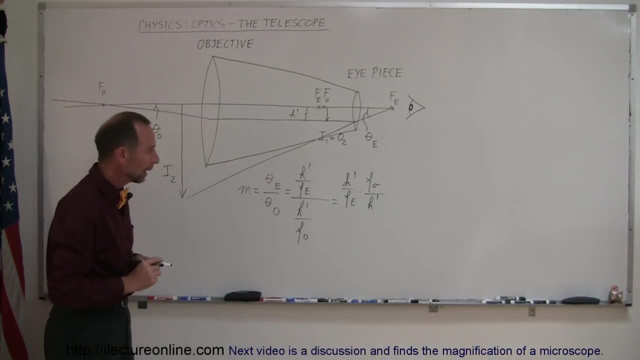 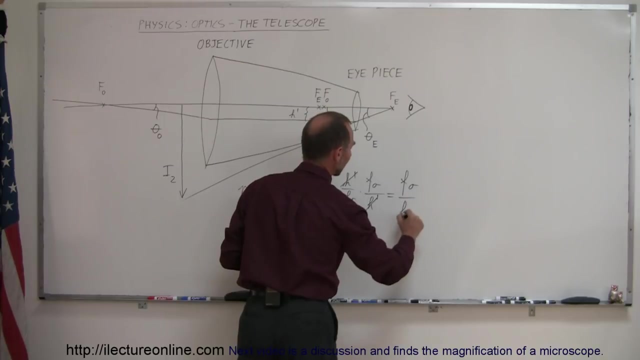 over f sub e times the inverse of the second fraction, which is f sub o over h prime. And then of course these cancel out, and then you can see that there's simply a ratio of the focal length of the objective lens divided by the focal length of the eyepiece, and that is. 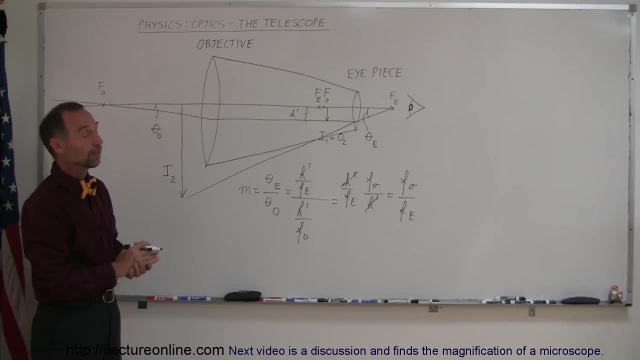 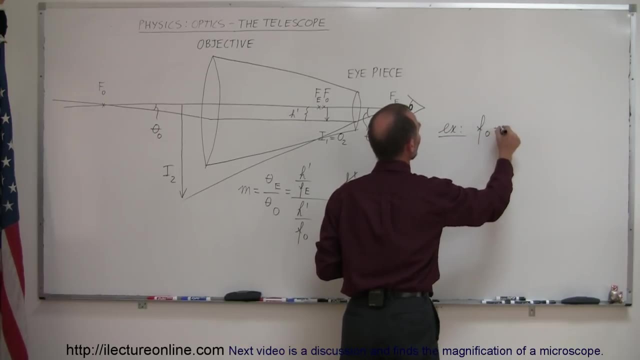 the magnification of any telescope. So that's pretty easy. So, for example, as an example, let's make it a little clearer Example. let's say that the focal length of the objective is equal to 150 centimeters and let's say that the focal length of the eyepiece